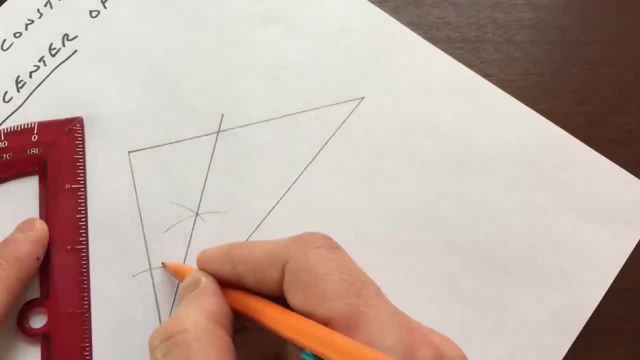 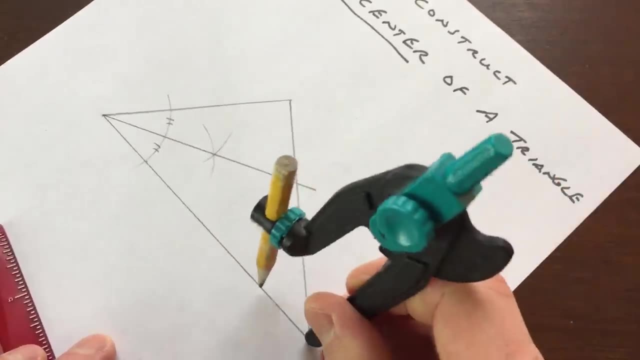 angle in half. okay, so you can see that this angle is congruent to this angle. So you're with me so far. So let's go ahead and go over to this other angle and let's do the same exact process. We're going to bisect the angle. so I'm just going to draw an arc and I'm going to 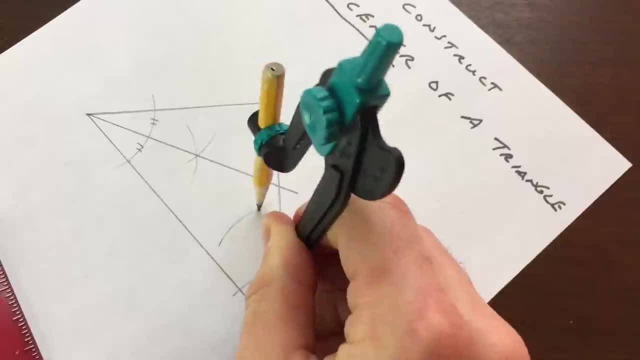 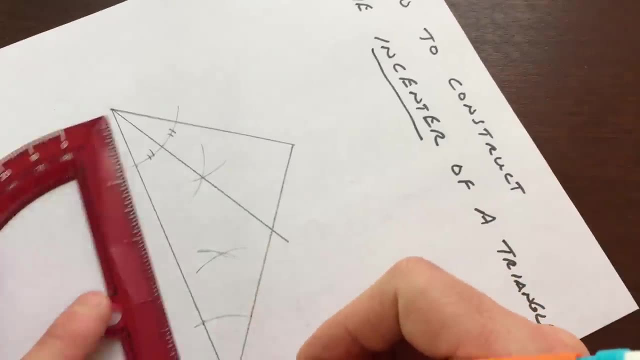 use these two points where it intersects the sides of the angle, and I'm going to draw two more arcs. Whoops, slipped a little bit there. Okay, there we go, and so what we're going to do is we're going to again draw an angle bisector from here to the point of intersection, like that. 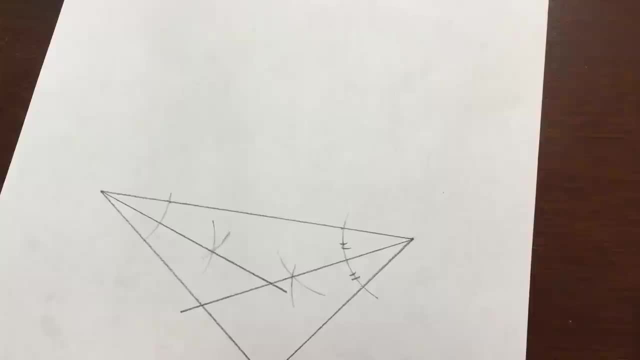 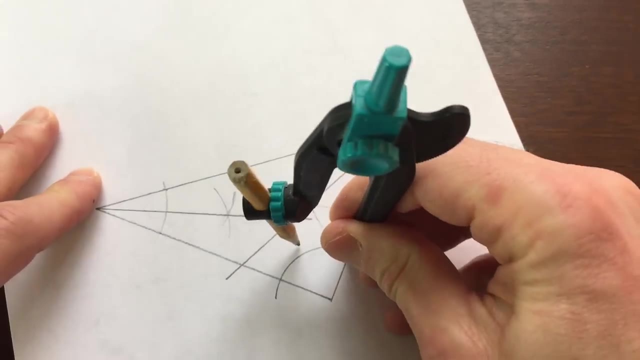 and then if we go ahead and go from this third angle, we're going to do the same thing. We find the angle bisector, so I'm going to go ahead and draw that in there and use the two points, open that up a little bit more. one: 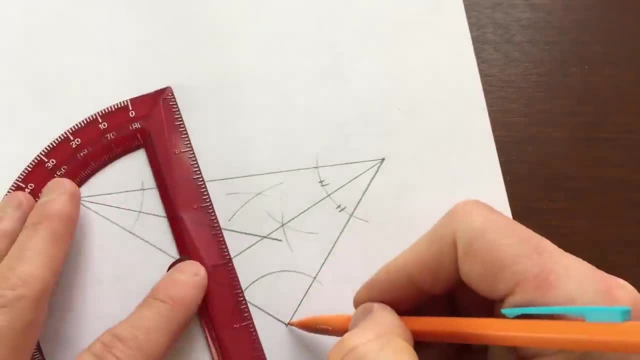 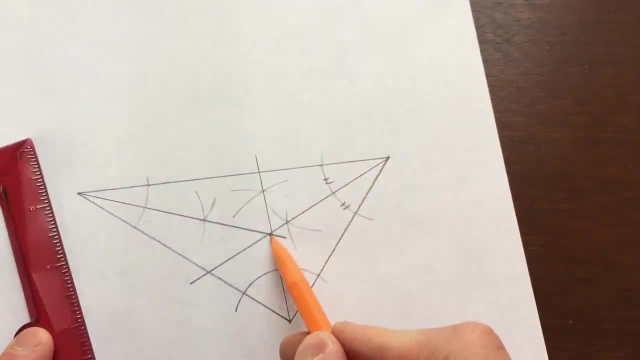 and two, and then what we're going to do is go ahead and draw a ray from this vertex through that point of intersection and you can see pretty, pretty close. You can see. that's where the three angle bisectors are. crossing is right here at this point. That's the in-center. Okay. 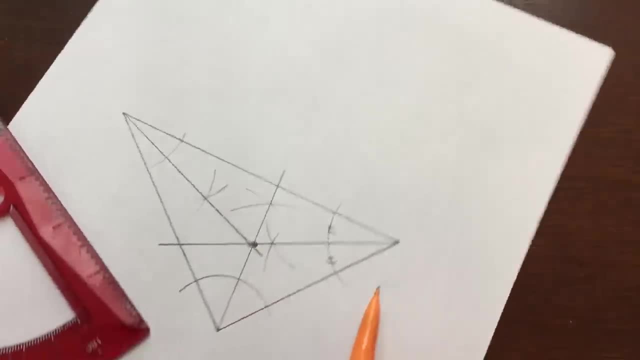 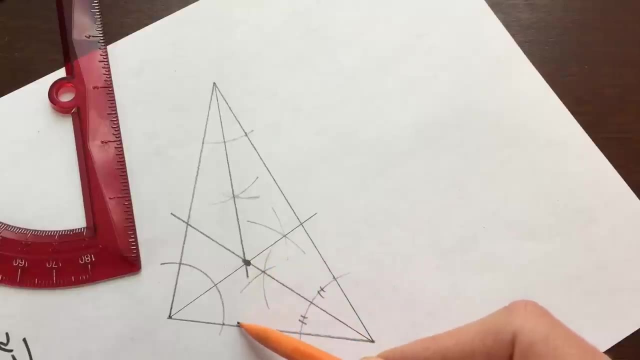 now the next thing we want to do- okay, to get an accurate drawing- is we want to find the shortest distance from this point to one of the sides of the triangle. Okay, that's going to be the radius of our circle, and what we're going to be doing is we're going to be inscribing a circle inside. 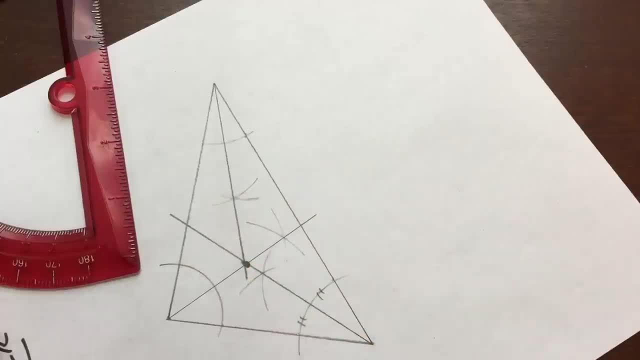 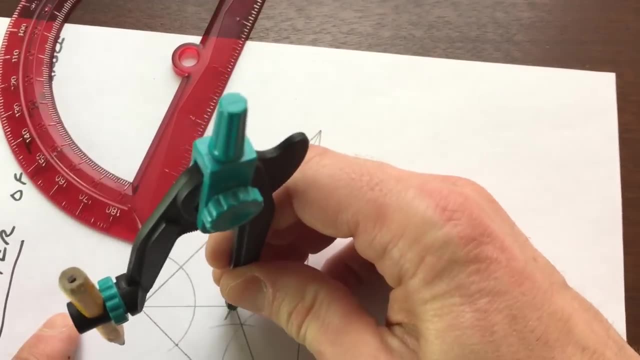 of the triangle, so it's going to just barely touch the edges of the triangle. so we want to be accurate about this process, so I'm going to use this point. I'm going to find the shortest distance, which is the perpendicular distance from this point to this line. so I'm going to go. 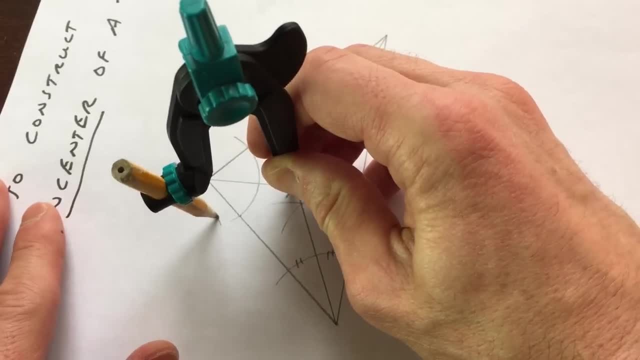 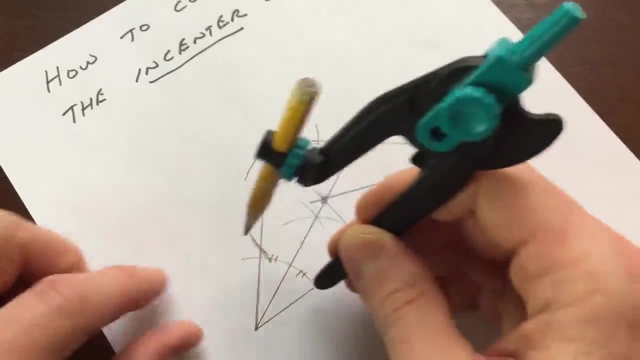 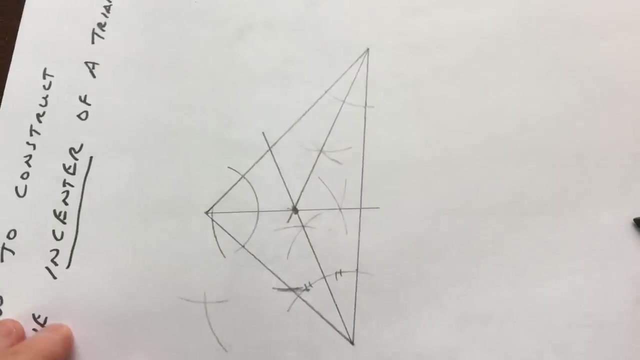 ahead and do that. I'm going to make an arc such that it intersects the side of the triangle- okay, at two points, okay there. and I'm going to use these two points to draw two more arcs, one and two, and then what I'm going to do is I'm going to draw a line. 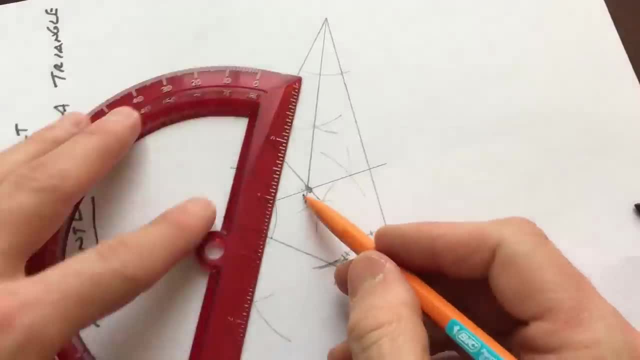 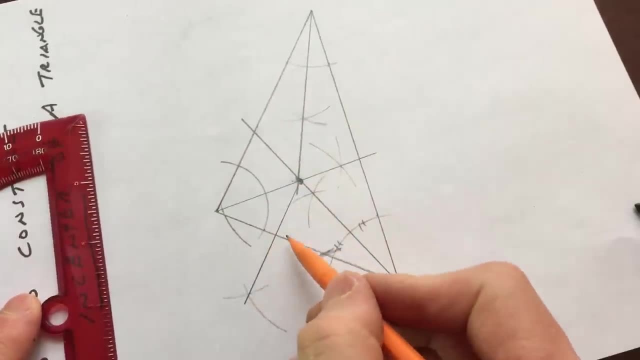 segment through this point and this point and that's going to be the perpendicular to the side of the triangle, so let me go ahead and do that, okay, so you can see that came out pretty good. This is 90 degrees right there, and then now what you want to do is you want to use your 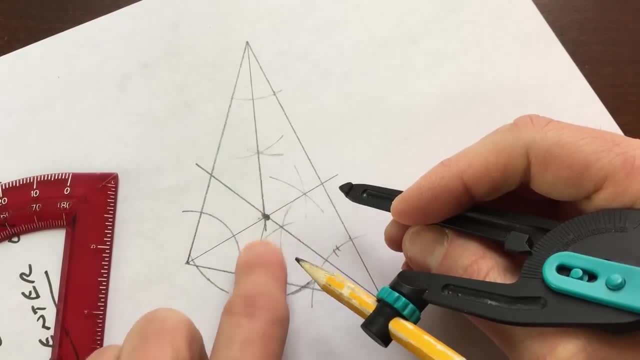 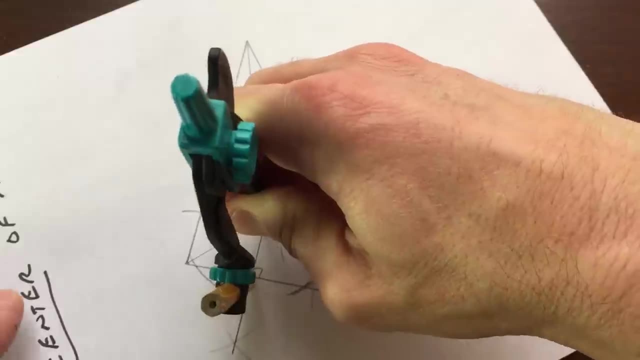 compass as a measuring tool. You want to open it up so that it's measuring from here to just the edge of the triangle, where it just barely- the circle is just going to barely- touch the triangle. so there we go, right there. so now what I'm going to do is I'm going to go ahead and draw the.